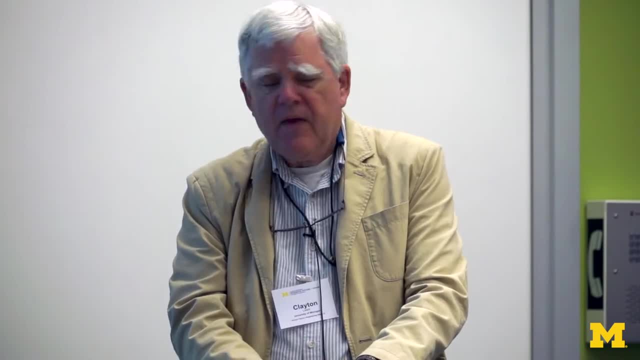 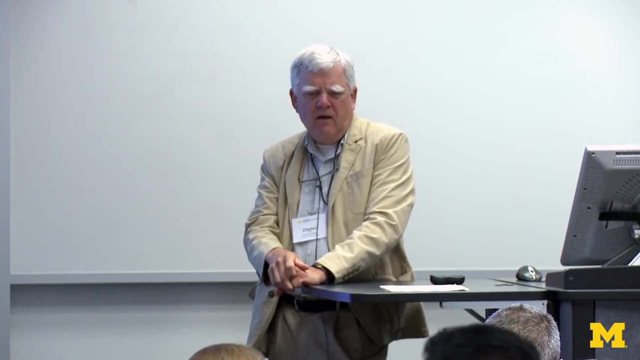 Is there reason to believe that the user will have an appropriate goal? If they do have the appropriate goal, will the interface make it obvious to them how they have to accomplish that goal? Okay, It could be clear what they need to do at this. 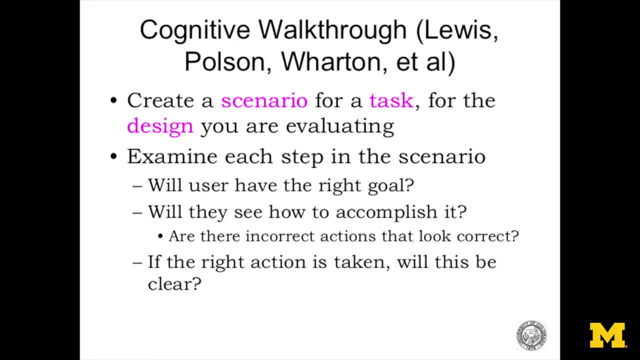 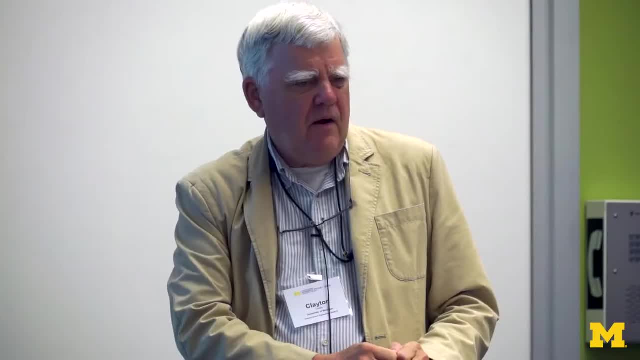 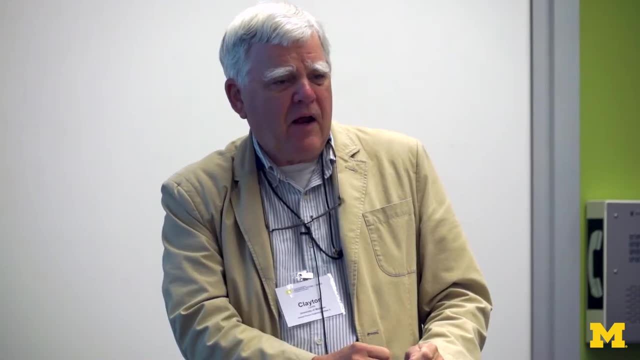 point, but they can't figure out how to do it, And it's something that happens over and over again. as a source of difficulty in interfaces is the person knows what they're trying to do. Maybe there's a button, label or something that really looks great for that step. Unfortunately, 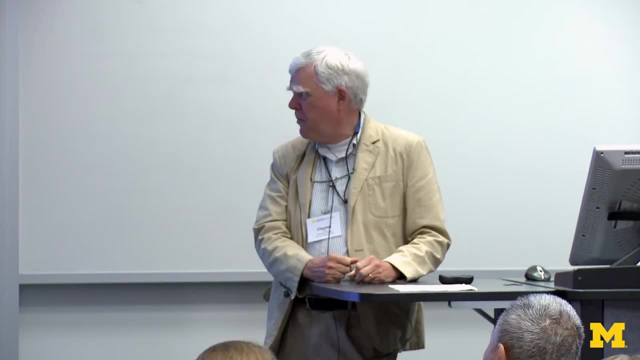 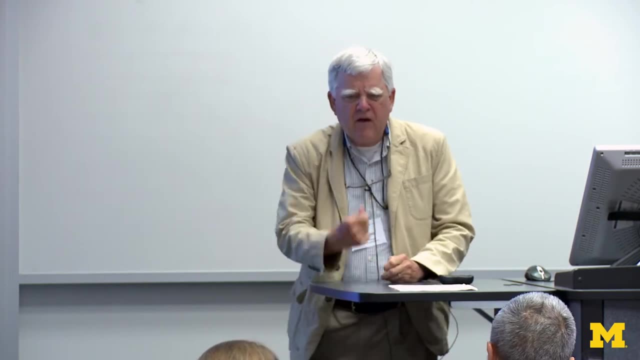 there's another button that looks equally great. That's going to be a problem. So if that's going to be a problem, then finally, suppose the person, they're on track, they're trying to do the right thing, they figure out how to do it, and then they do it and 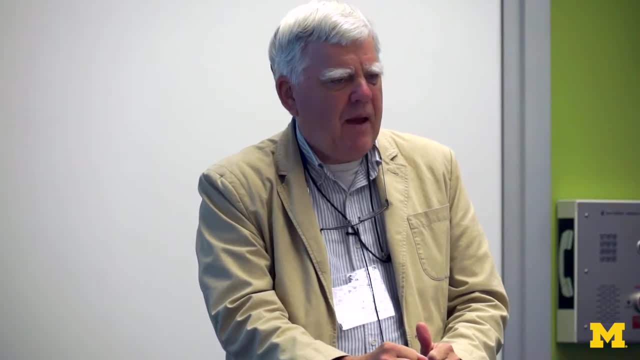 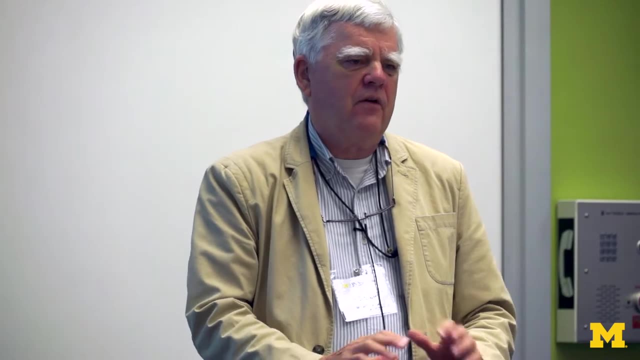 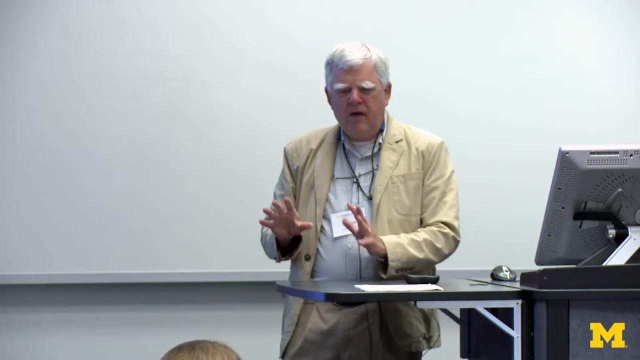 something happens that looks weird. It's not what they expect. They say, ooh, I thought I did the right thing, but obviously I didn't. I'd better back up and make another choice, Big trouble. So those are the key evaluative questions that you're going to ask yourself. 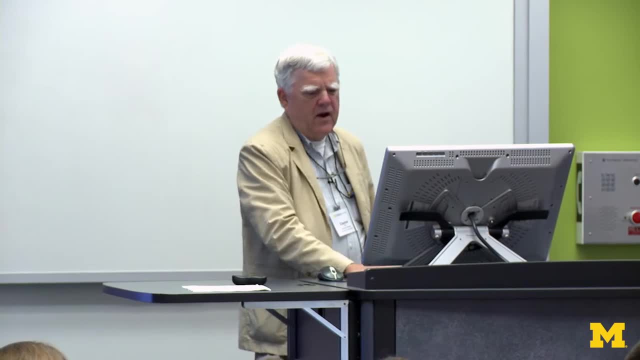 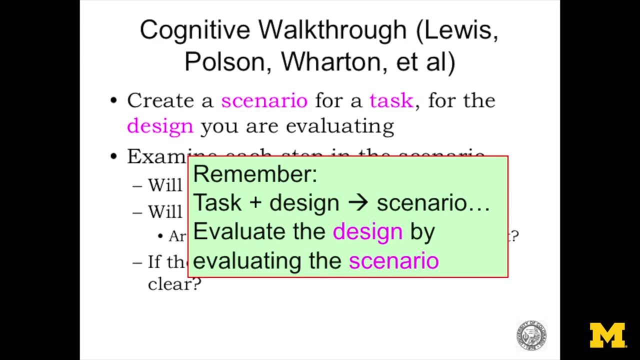 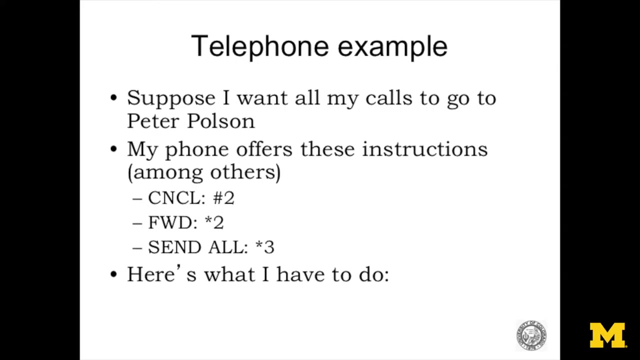 as you look through each step of the scenario. So again, what's happening at a high level here is we're evaluating the design by generating a scenario for a particular task and then critiquing that scenario. So here's a real world example. This is the way the telephone on my desk still works By now. it's a pretty 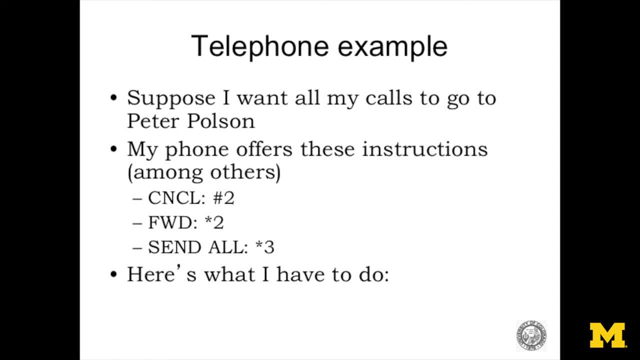 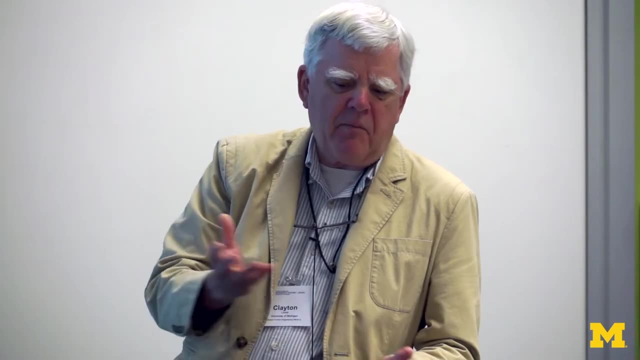 old system, but telephone equipment never wears out, So this is still what's happening back home. So I've got a phone and one of the capabilities it has is the ability to pass my calls on to a colleague if I'm expecting an important call but I'm not on hand to take it and I 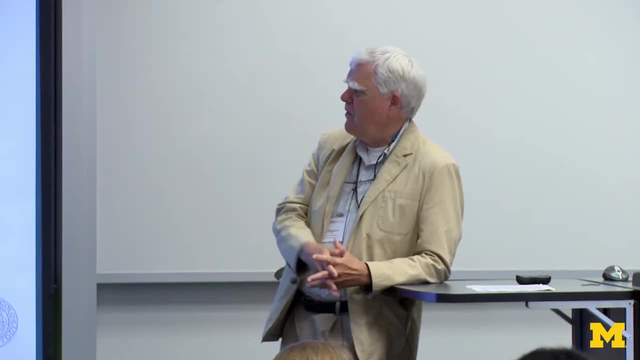 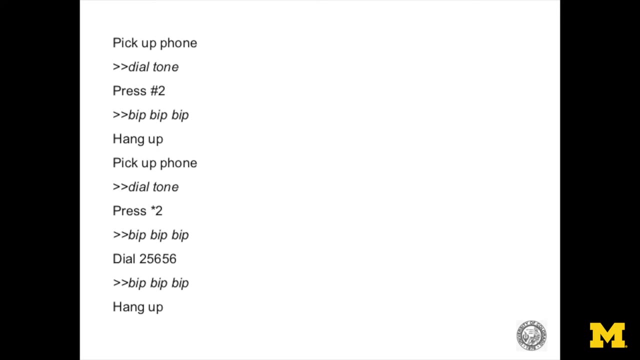 don't want it to go to voicemail. I could arrange to have, for example, Peter Poulsen pick up that important call and deal with it. So here's what I have to do to actually perform that operation, And the things with the little. 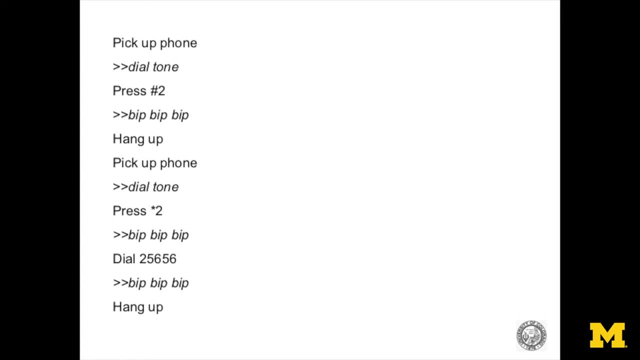 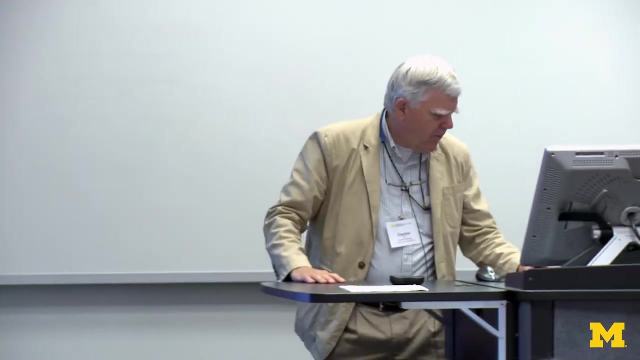 angle symbols there indicating audio responses that the phone makes when somebody carries out the preceding action. So I pick up the phone and I got a dial tone, But what I'm supposed to do is to press pound sign 2.. Actually, as we go through this, it'll be helpful to 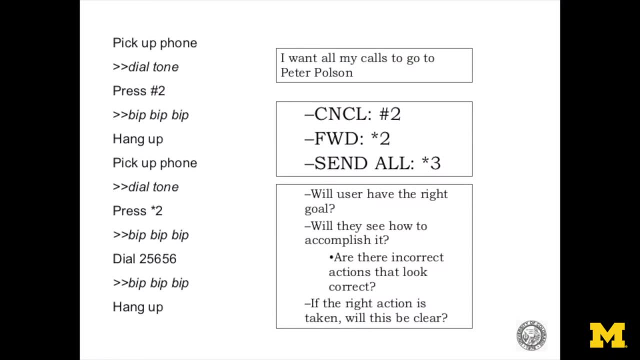 as a reminder, here have the information on that overlay that somebody might use to figure out what operation they should perform here. So I've got to perform that pound sign or number sign 2 operation. If I do that I get a bit-bit-bit tone. Then I need to hang up, Then I need to pick up the phone. I get the. 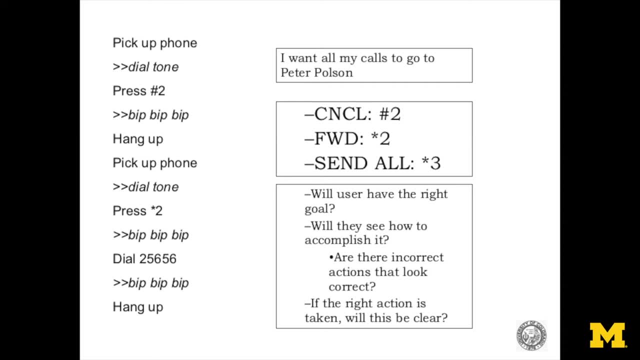 dial tone again, Then I'm going to press star 2, and I'm going to get another bit-butt-bip, And then I'm going to dial the indicated number. there I'm going to get another confirmation, Then I'm going to hang up. 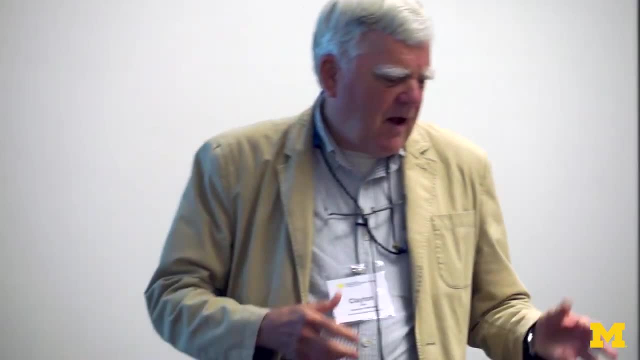 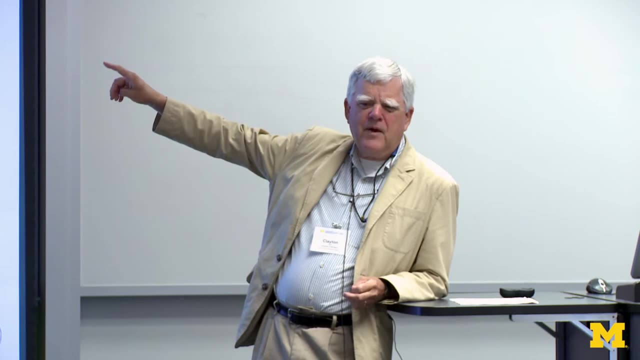 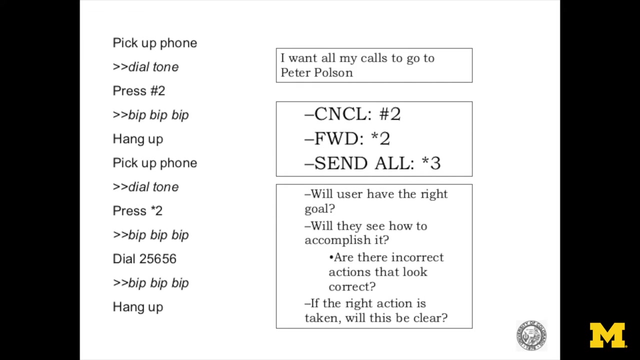 So, before we dive into this in more detail, some of you may be understandably a little bit baffled. I'm going to give you a little bit more detail about what that pound sign 2 thing is doing up there. Well, and you can see that the template tells us that pound sign 2 is CNCL, And maybe you 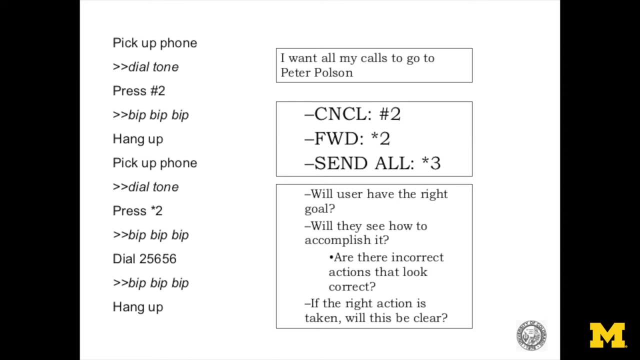 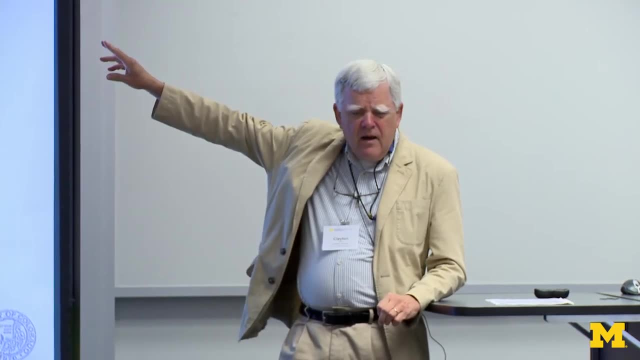 can guess that that means cancel. So here's what we're going to do. So, actually, the first thing is- and this is an important point- as a designer, what you're going to do is to lay out what you hope users are going. 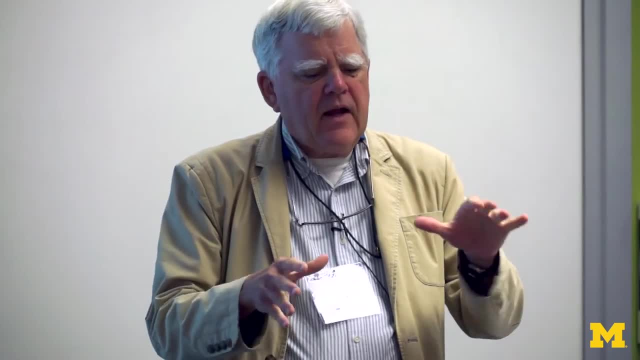 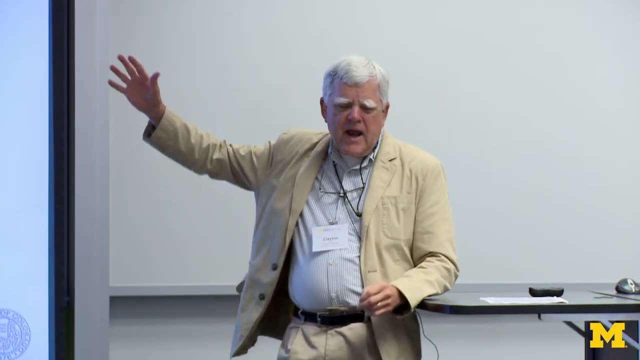 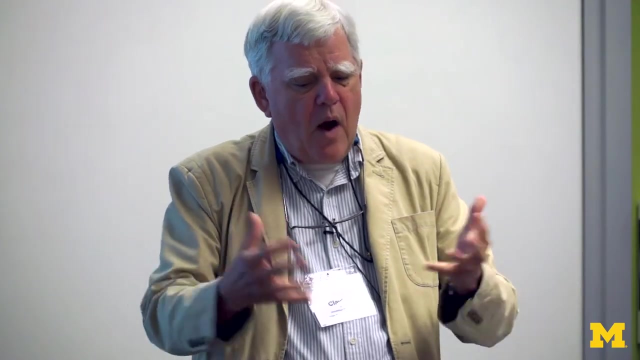 to do OK. And then you're going to ask yourself: is it credible that they're going to do that thing? that I hope So. you might ask: well, where does this scenario come from? Well, you're the designer. You generate the scenario based on what you had in mind in. 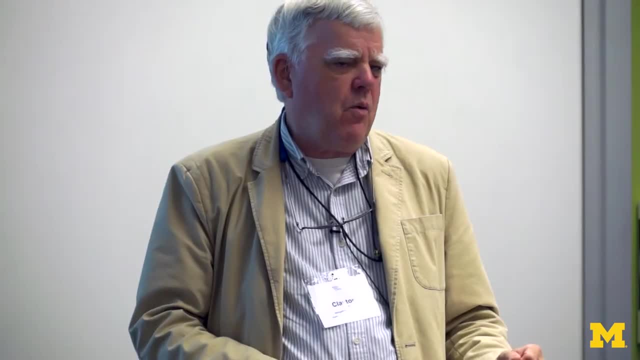 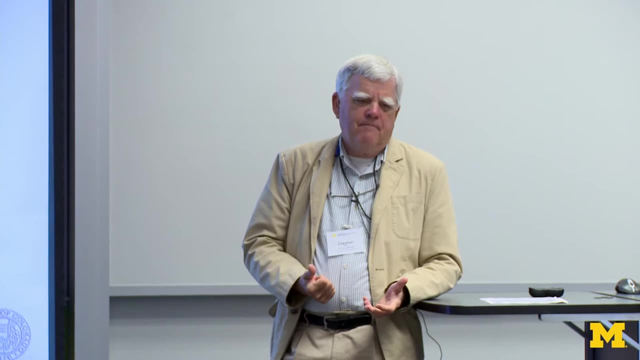 designing this. So if this is what you expect people to do, that's what you want to critique, because what you're trying to ask yourself is: will this actually work the way that I hope it will, OK, So So let's just stipulate that this is the way it's supposed to work. 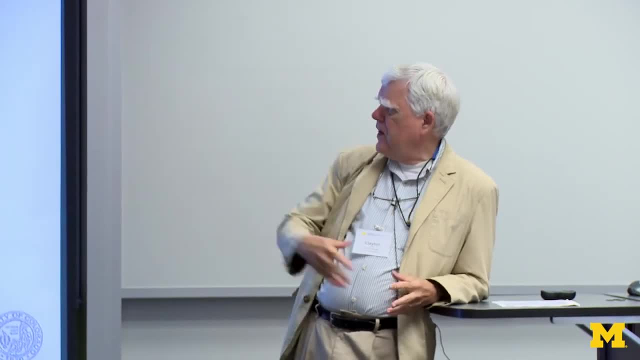 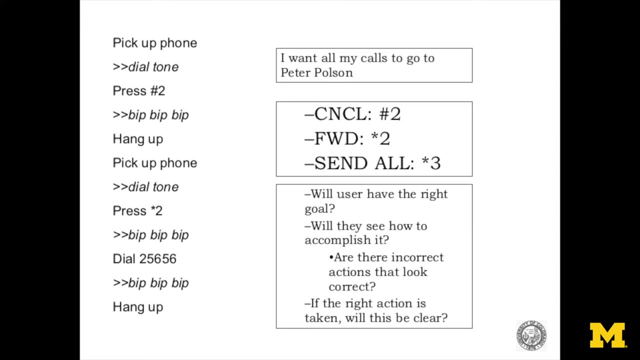 And now we're going to go through and we're going to ask ourselves the key questions here about each step. So how about that first one, picking up the phone? Will people understand that that's something that they need to do? What do you think? 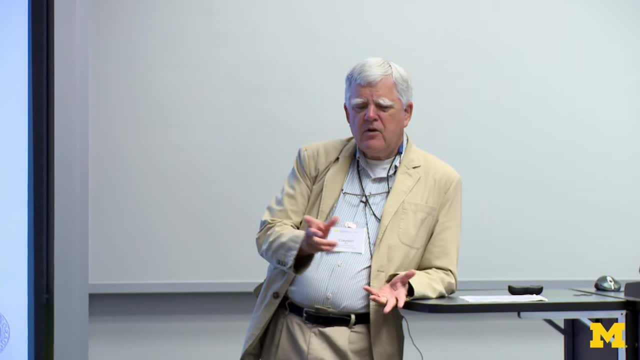 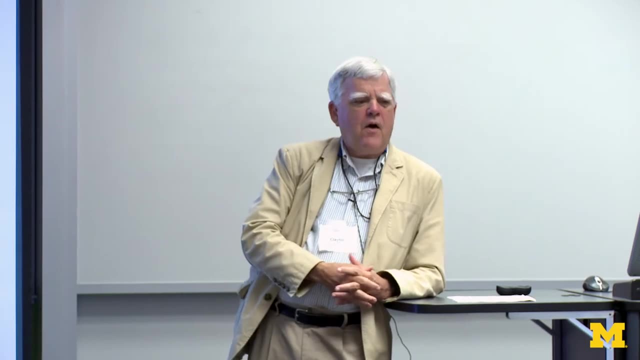 I hear a lot of yeses. I see a lot of nodding. I'll just note- and you may have had this experience, I think many of you will have- It used to be that a pick-up-the-phone step like that was a complete no-brainer. 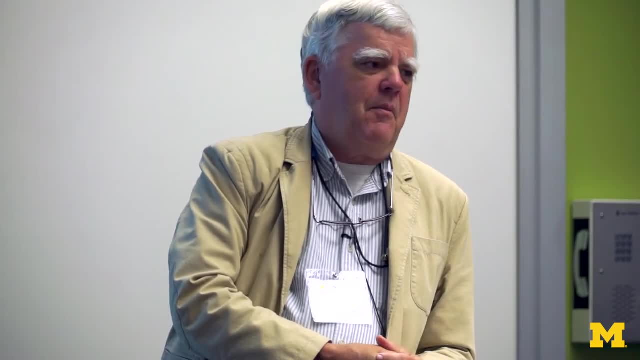 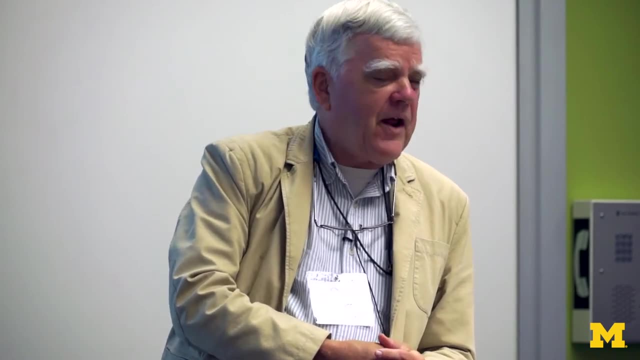 Because the way phones used to be, they didn't do anything until you picked them up. But if you've noticed, a lot of phones don't work that way anymore. There's lots of things you can do on the phone without having to pick it up. 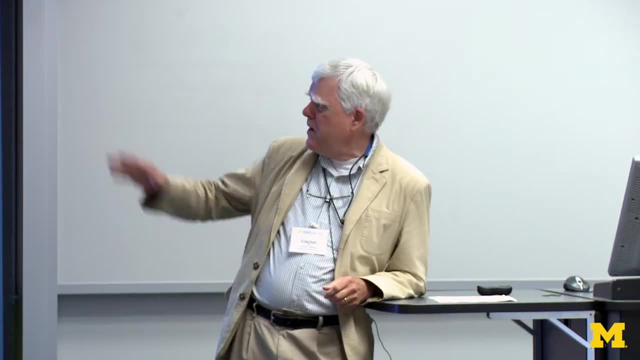 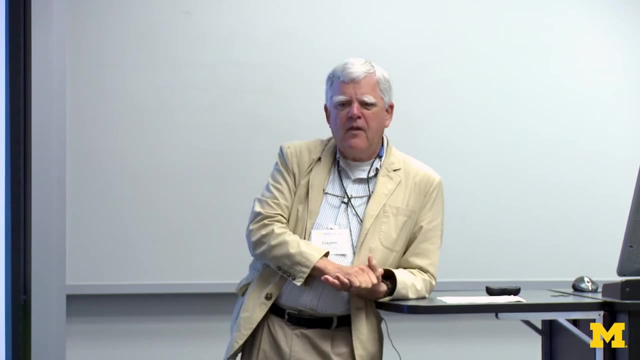 And in fact I would venture that you can probably find a phone where you can perform this operation without picking up the handset, Because you know they've got buttons and displays and they've got all that kind of stuff. Phones are way more complicated than they used to be. 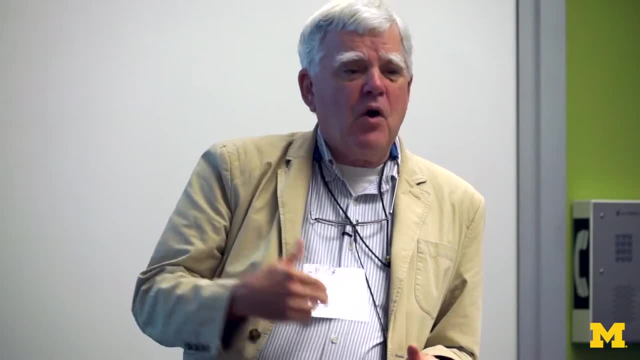 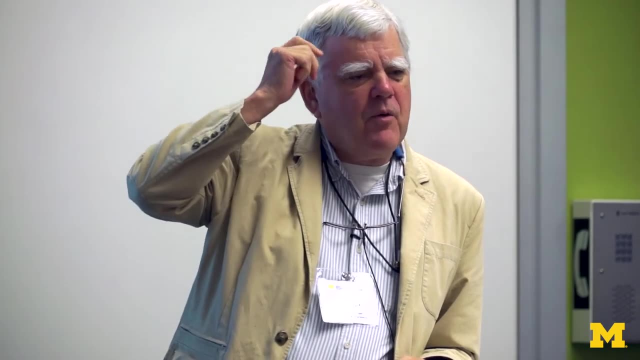 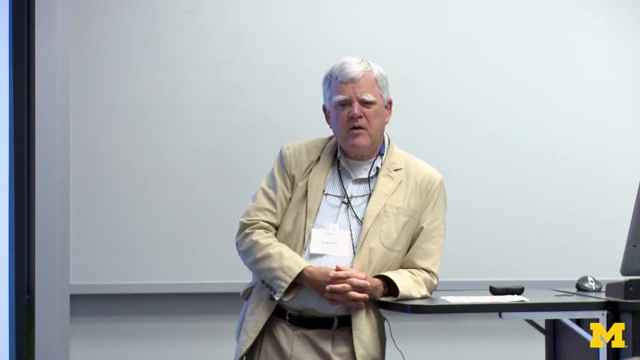 But at least for this audience, this demographic here, you're okay with the notion that people realize. yeah, I've got to pick up the phone before this happens, But you might register somewhere in your head, maybe against the time that you're going to be doing user tests with this design down the road. 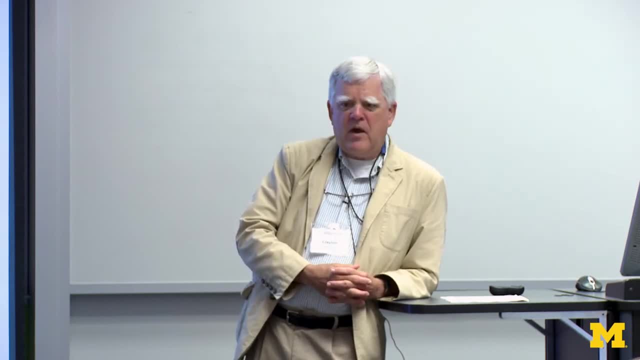 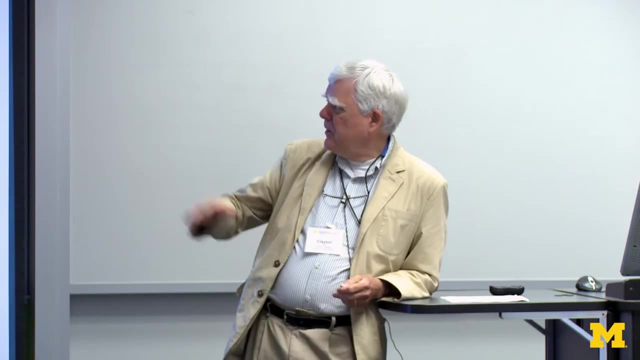 you might be saying, well, let's watch that, Okay, and let's see whether we find people starting to press the keypad before they've picked up the handset. It could happen, But let's pass over that one, Okay. then the phone responds with a dial tone. 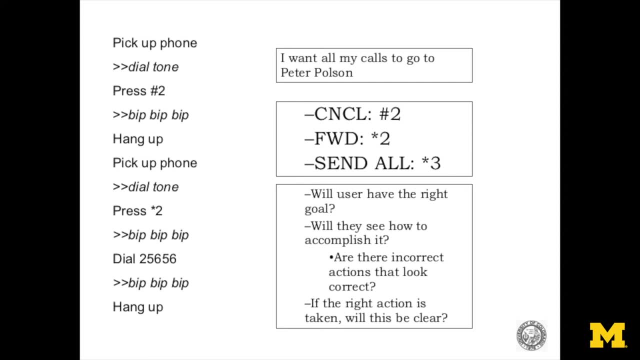 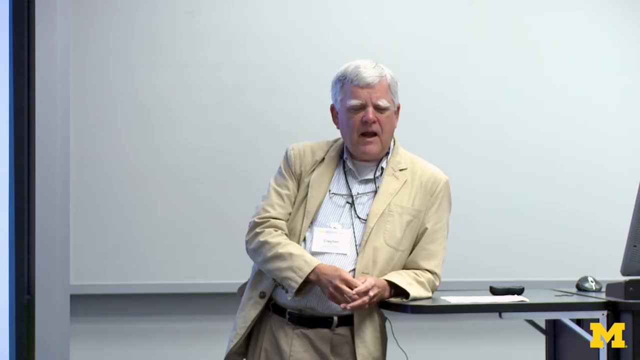 Remember the question there is: when you take the right action and the system responds, do you feel good about what's going on? And I'm going to venture that probably everybody, or nearly everybody, in the room would say: yeah, dial tone. yeah, that's what you expect phones to do. 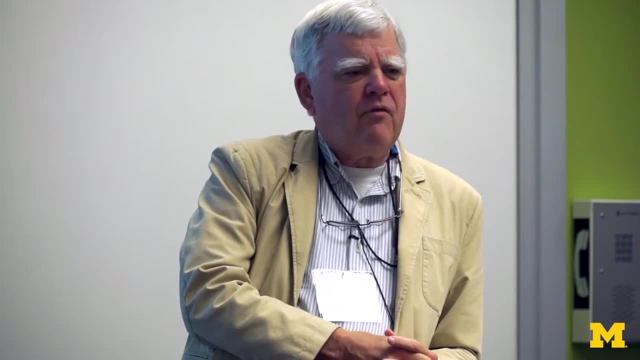 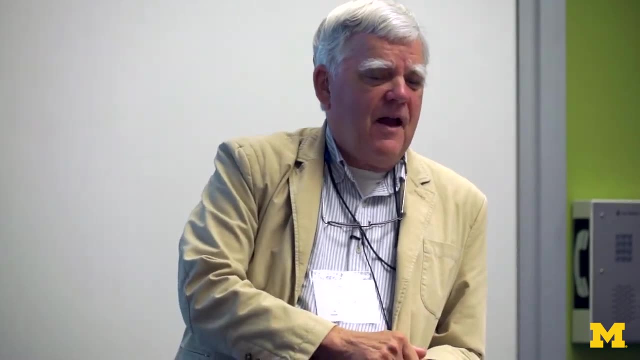 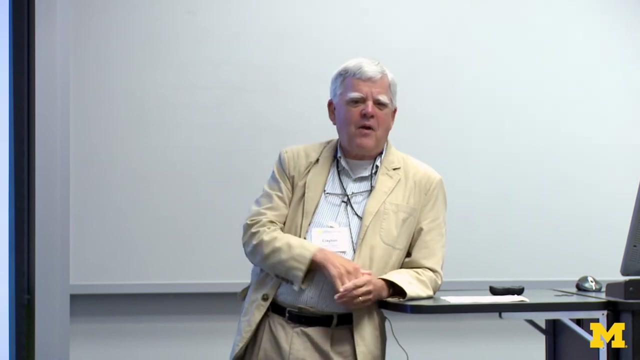 So I'll just note- maybe some of you had the experience. I've seen a lot of people using phones in another country. They have their own set of tones that are different from ours, And at least my experience is. frequently the phone makes some noise and I have not the least idea whether that means yep, you're on the right track. 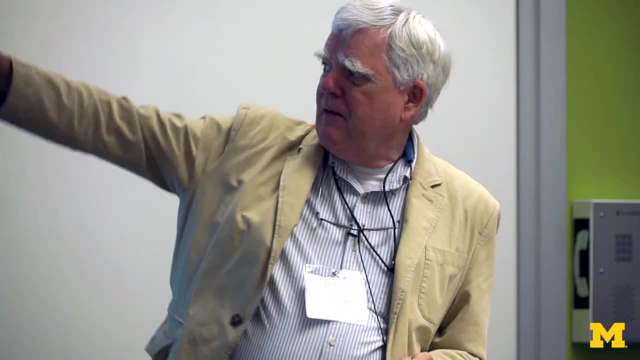 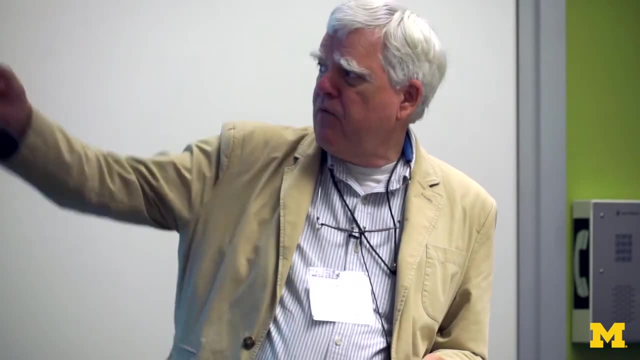 or whether it means: hey, what are you trying to do, buddy? Okay, but again, let's pass over this. But if you were designing for an international audience, the stakes would be higher here. You could ask yourself: why is that tone going to mean anything? 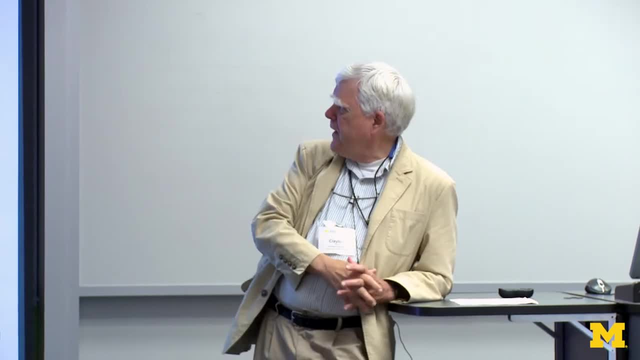 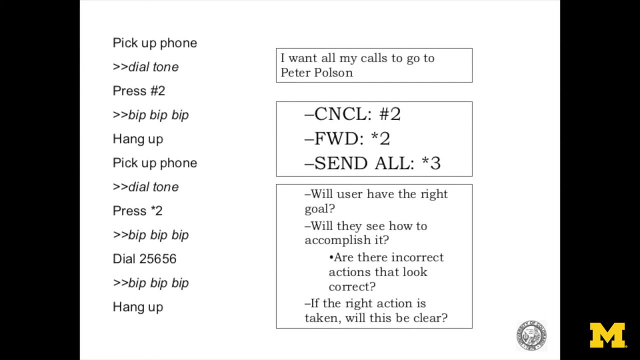 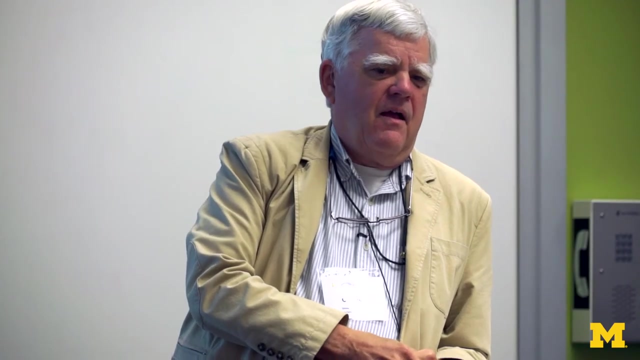 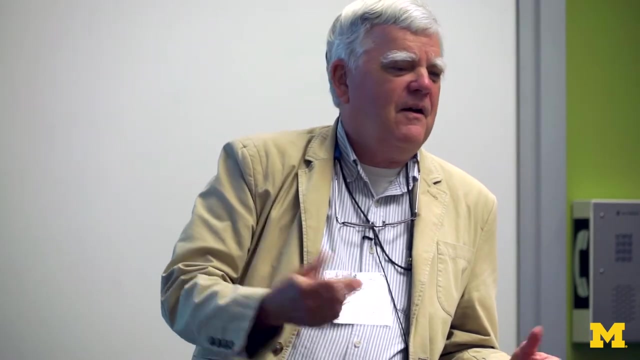 It's just a tone, But let's pass. Let's pass over it for now. Okay, then we get to that press pound sign too. I've already really raised the point about that. I think we can all agree that nobody is born knowing that. well, of course, the first thing you have to do when you're transferring your cars is to make sure you've canceled what's in there before. 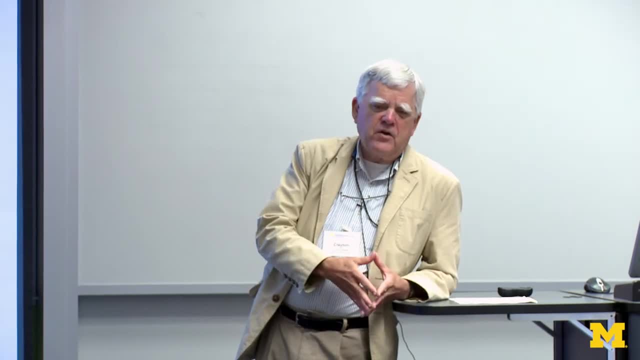 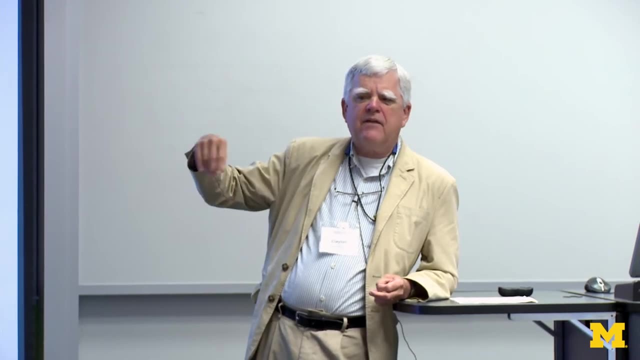 Nobody's going to know that. So, as I've already told you happened to me. that's a real Gotcha. Okay, and notice, it's not that if I knew I had to cancel, it would be hard for me to figure out how to do it. 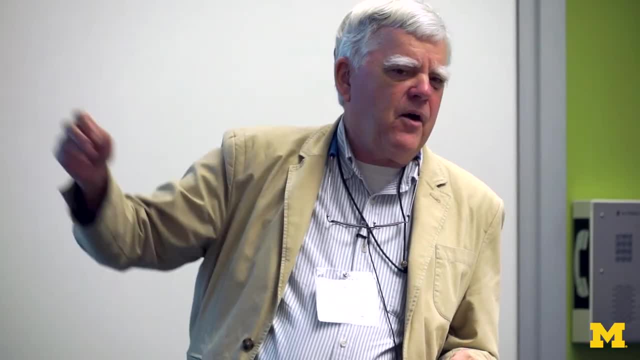 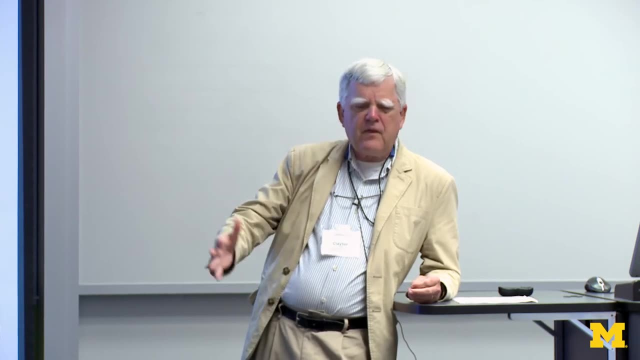 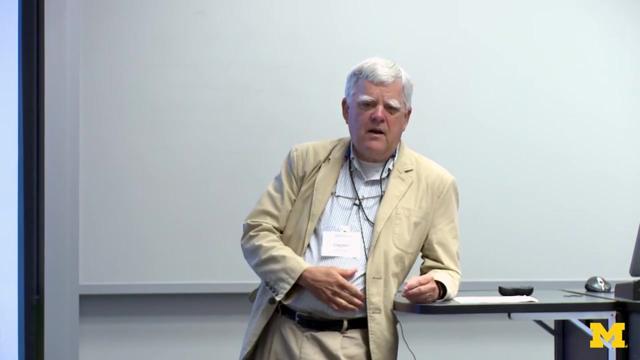 I mean, maybe the abbreviation is a little cryptic, but probably I could figure that out. The problem here is it's an unmotivated step, I don't know that I need to do that, And so that's something that training or one of those other things that should be a matter of last resort is going to have to come in on. 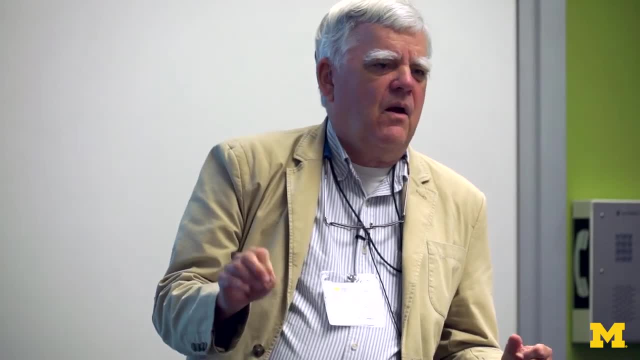 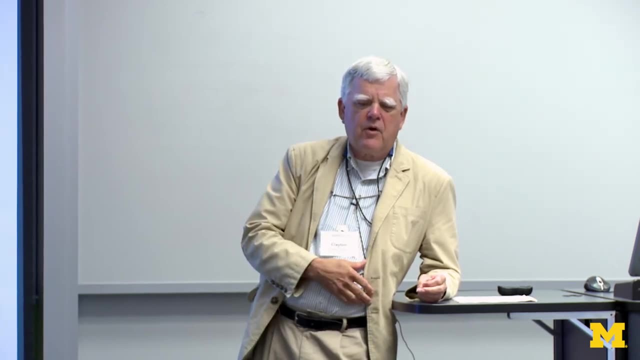 Again, there was no doubt was some good reason Why The system was designed to have that particular failure mode where failure to cancel led to a failed transfer operation. I don't know what it was, but that's a big, that's a big issue. 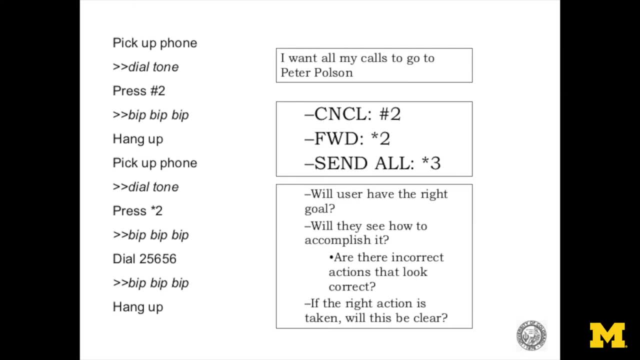 I think we can all agree. Next, Oh, then we got the bit bit bit- Same kind of comment there, The bit bit bit, which is used consistently in this interface. In the designer's mind, the bit bit bit is a confirmation. 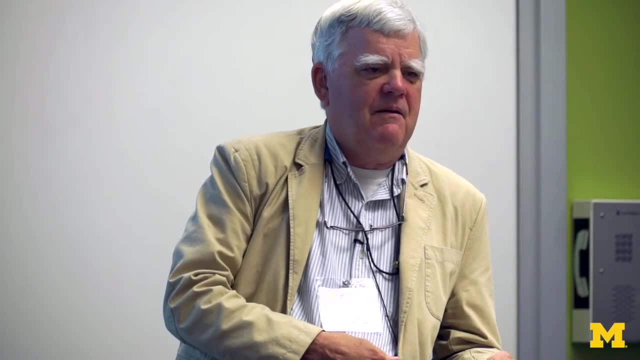 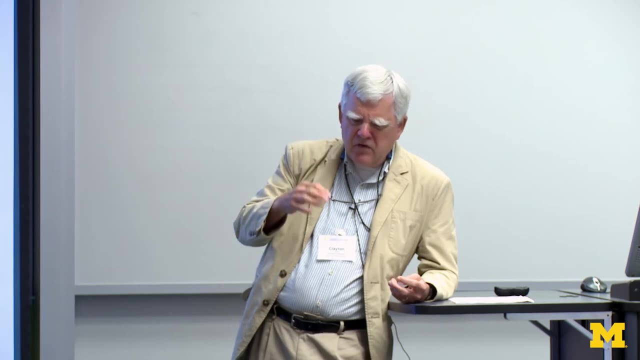 That means yep, I got what you did. First time I heard it it didn't mean anything to me, but you know I kind of got used to it again. We can register that gee using these cryptic sounds: 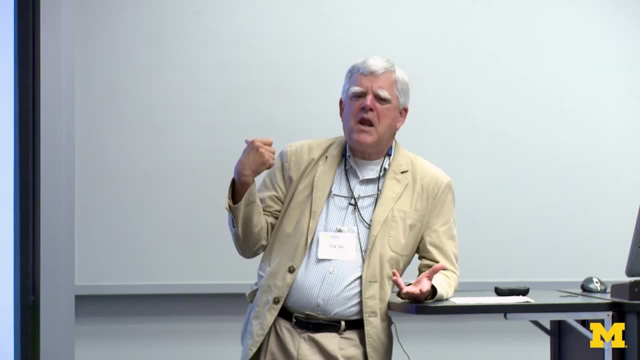 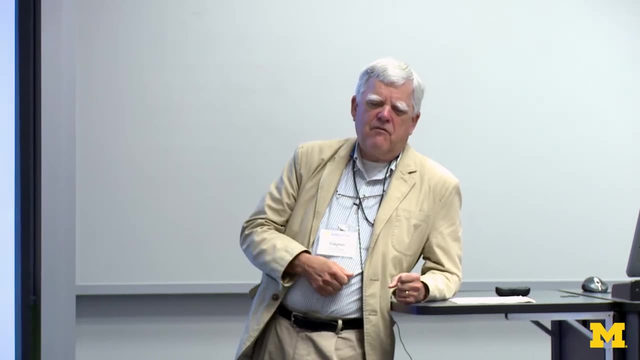 Can we do better than that? And you know, for this phone hardware, maybe not for a phone with some kind of display capability? Almost certainly. yes, you could do a better job in giving a person an idea of what was going on. 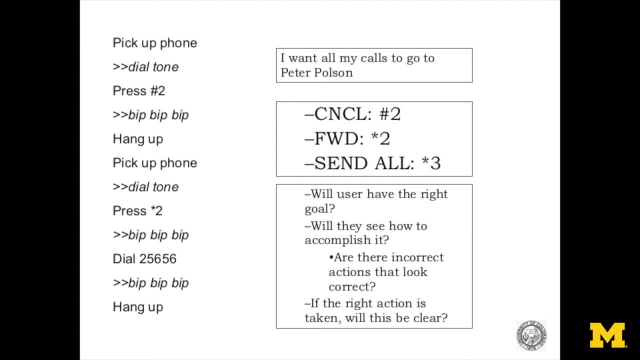 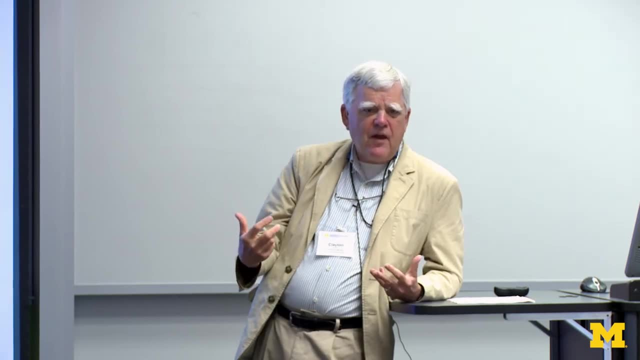 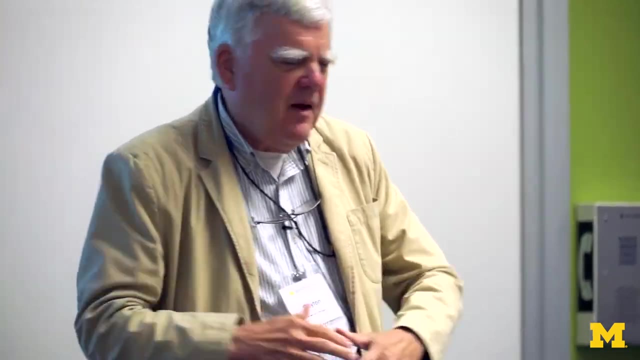 Next step. there Hang up. What do you think about that? Any comment, Totally unmotivated, exactly. Now again, whoever designed this thing could probably explain. well, Clayton, you have to understand. the phone is connected to the private branch exchange or whatever it is. 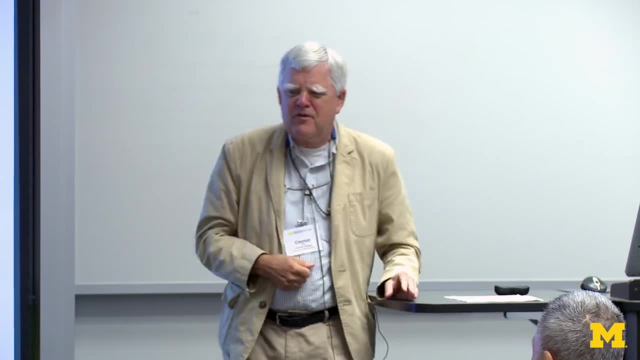 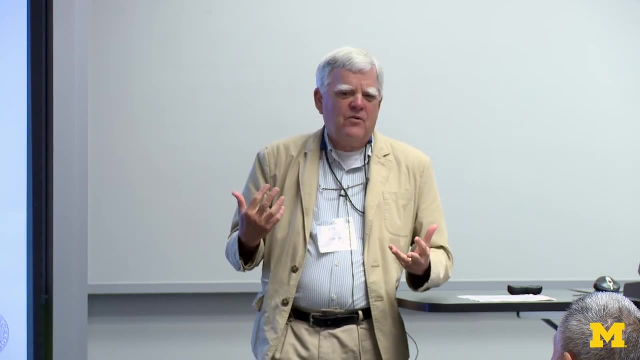 and the private branch exchange needs that hang up to terminate the such and such transaction, And my response is: I don't want to know. okay, But more than that I don't know. So I have no way to know that I need to hang up at that point. 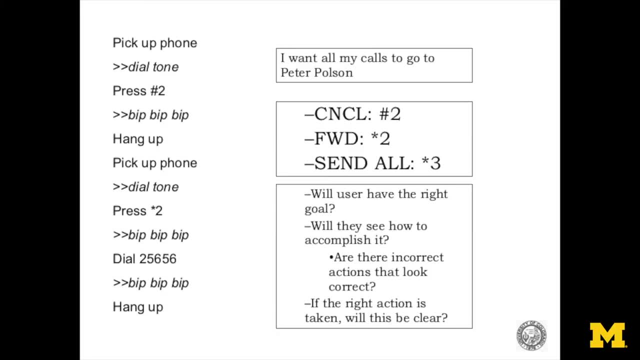 Okay, pushing on. we've got to pick up the phone. We've already covered that thing. We've got the confirmatory dial tone. Now look at the next step. there Press asterisk 2.. Forward is the word that the design uses for what we're doing here.